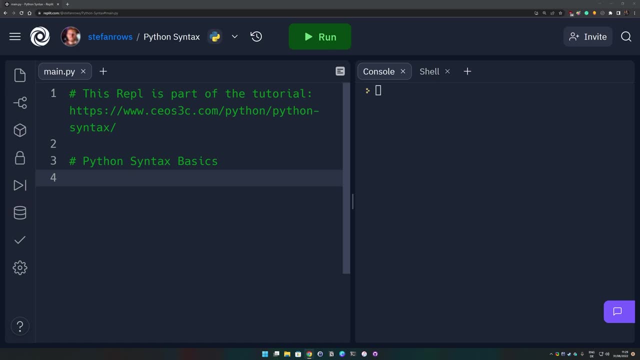 as JavaScript before. you probably have seen that certain statements are ended with a semicolon like so. So this is not the case in Python. In Python, everything is structured using white space. It is up to you if you want to use spaces or tabs, which kind of is an ongoing discussion. 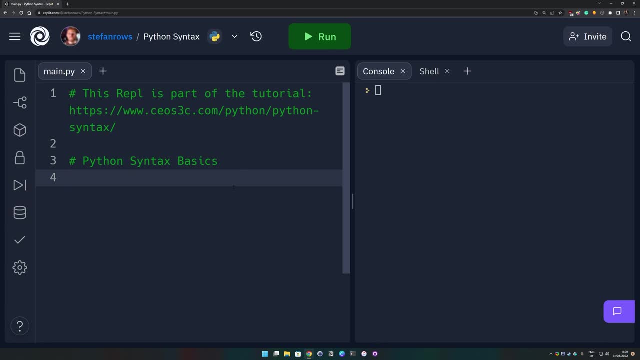 between people who prefer tabs over spaces or vice versa, But it's really personal preference. We like to use tabs because it keeps everything more uniform. But do note: if you use spaces according to the official PEP 8 style guide, you should use four spaces for indentation. 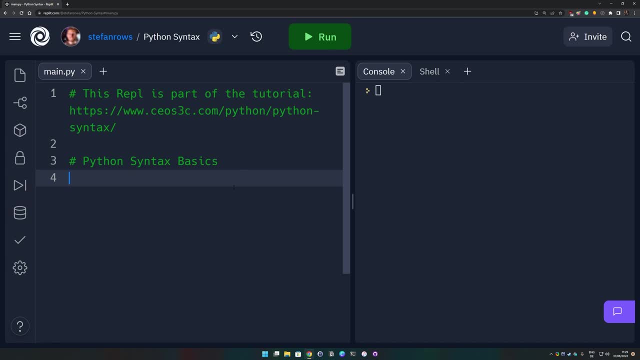 If you use tabs, just one tab is fine. You should never mix spaces and tabs, Always stick with one. So if you use one tab here, that's one tab. But if you actually look at four spaces- one, two, three, four- that's a bit further in an indented, But that's fine. if you use tabs, which we do recommend you for- 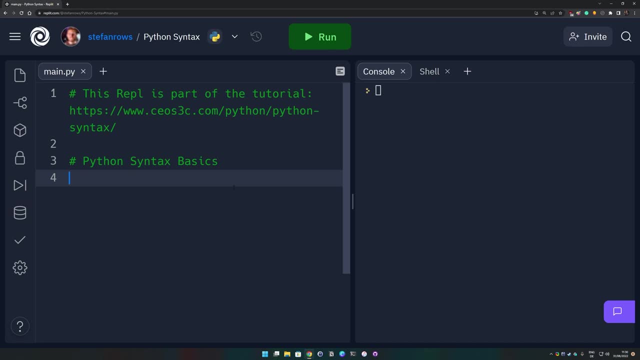 ease of use, then one tab is just fine. So let's look at an actual Python code snippet Now. don't worry about any of the things that I'm writing here. Don't need to understand that. it's simply about indentation. If you create a function in 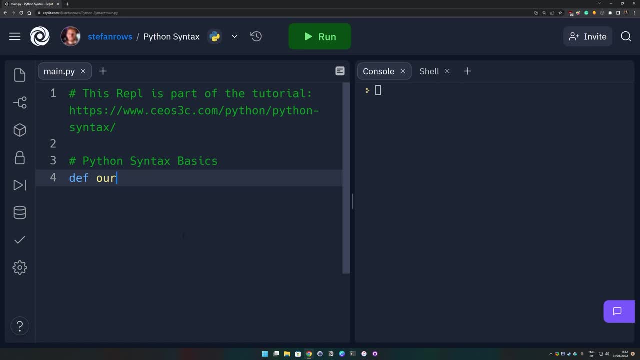 Python we use the def keyword and then we do the name of our function and then we do parentheses on the end and a colon, and then we do a print statement here And you can see, while I was pressing enter here it already automatically indented our code, which means that we are now. 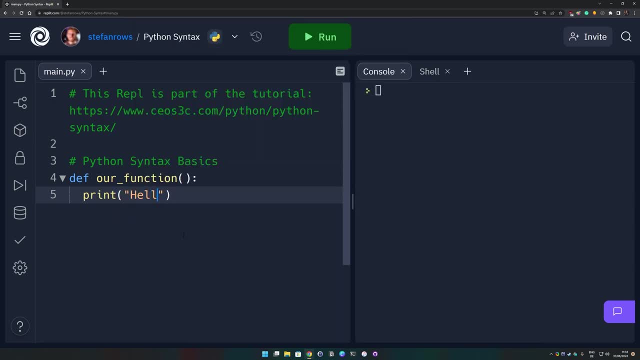 working inside of this function. So we do hello from our function. This is a simple print statement. You will learn more about this later. Again, this is only about the structure of the code. And now if I hit enter once more, then I'm still inside of this code block. And if I hit enter, 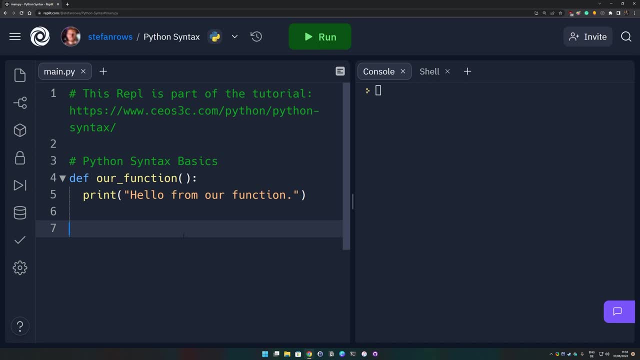 once more, at least here in REPLIT. every editor is different, but most of them have some form of auto indentation And that's how you can work. And if you want to actually get back into the function, you can just go back one step up and then press the tab key and you will be in the exact same line here. 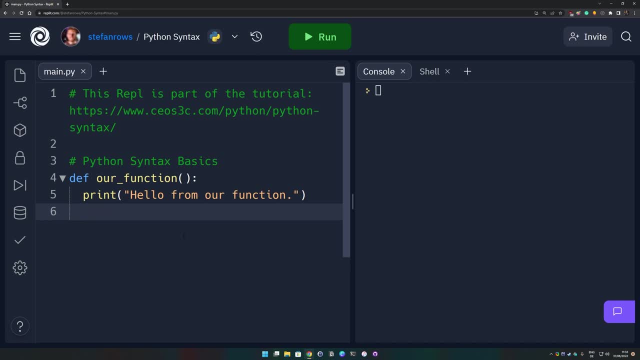 And this is exactly what we're doing here. And if you want to actually get back into the function, you can. so this is the indentation. Now, if we actually want to call the function, we do our function and parentheses on the end, And then if we run our code, our code will run and print the statement. that's. 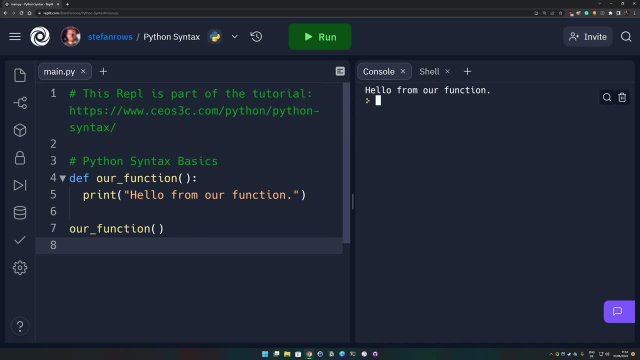 coming from our function. But again, don't focus on what is all of that here. Just focus on the indentation part And you can see that this is clearly indented one tab in. You may also recognize that we don't need any kind of semicolon at any stage. We don't need any kind of semicolon at any stage. 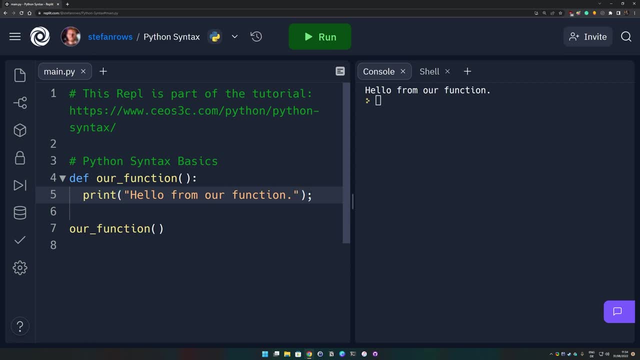 the end of our function statement or of our print function here we don't need any of that. so this not only allows us to write less code, but also makes it more of a human readable language that actually reads a little bit like english. to summarize here why or what are some advantages? 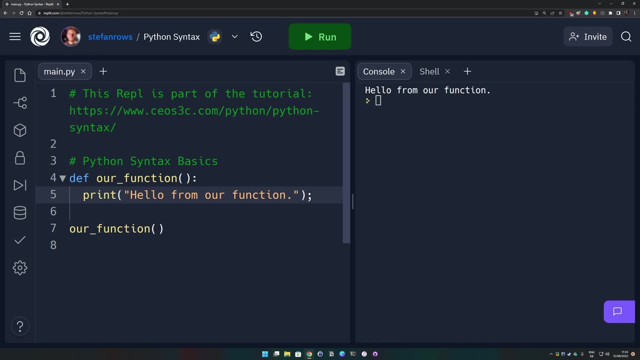 of using this approach there is better readability, clearly defined functions by using indentation. indentation is required, which makes reading other developers code easier. so if you jump into code of some other developer that you haven't been working with before and it's all correctly indented, you can. 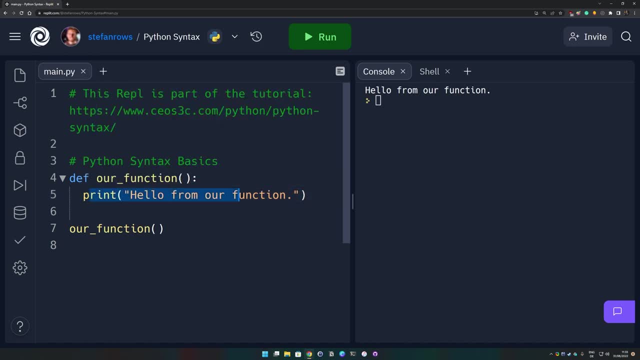 directly see that this is part of the function, and if it would be indented that way, you would see that it's actually not in the function and that the function is empty. so once you develop a little bit of an eye for that, then you can better understand why we indent code there is. 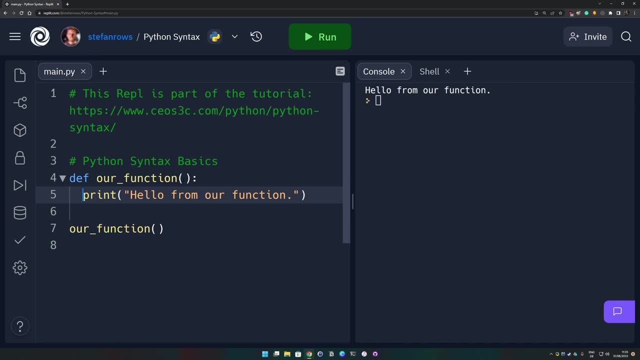 also a lower barrier of the indentation of the code. so if you have a function that you want to indent code, then you can better understand why we indent code. there is also a lower barrier of the entry. It makes learning Python syntax easier compared to other languages. So 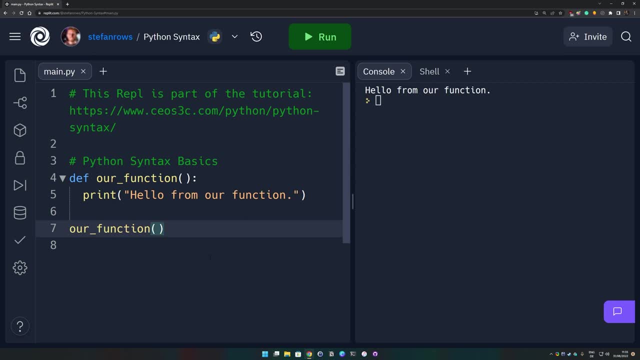 all of that green syntax you see up. here is a comment, and comments are essential in programming. Let's write another comment down below here. So this is a single line comment in Python and it won't run if you execute your code. Comments and programming languages are an essential tool to describe your 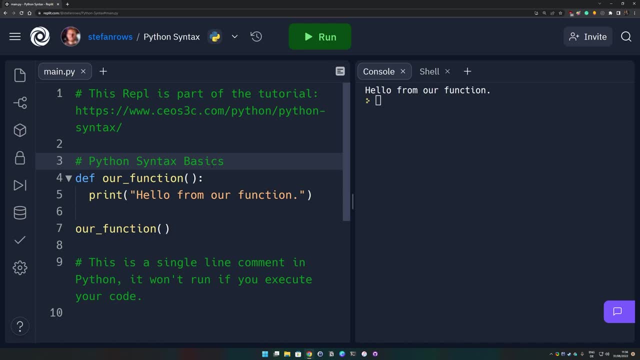 code, not only if you work together with other developers, as previously mentioned, but also for yourself. if you have a project that you haven't been working on for longer periods of time, you will forget parts or somebody else that can be applied to a borrow problem, So don't be afraid to. 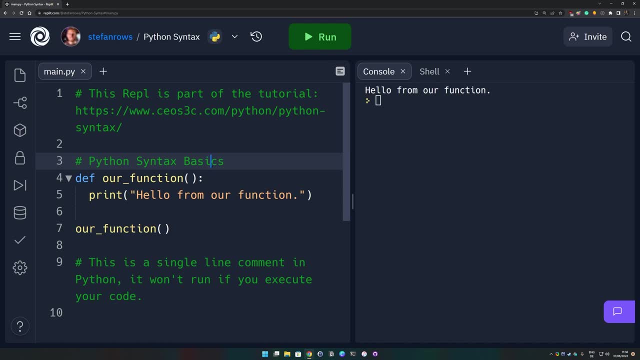 Sometimes all of it, all of its functionality Comments help us to remember what we have written and with pointing out key elements of our code's functionality. Writing comments is required in most programming related jobs, since you almost always collaborate with other developers on different projects. 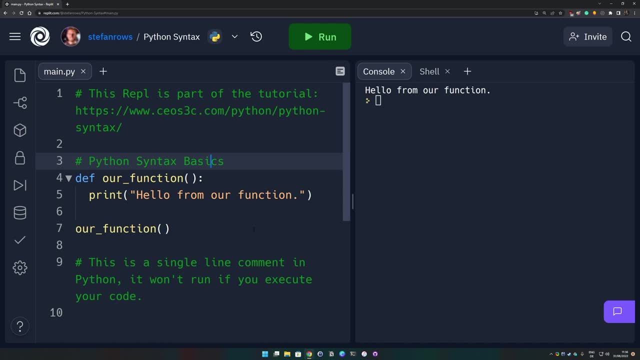 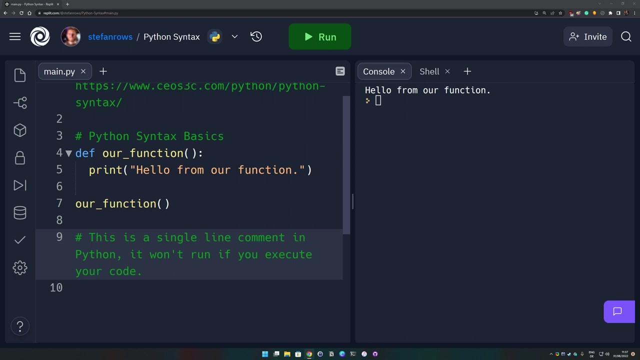 Commenting in Python is straightforward. To write a comment, you simply put a hashtag in front of your comment, like so, and this indicates a comment to the compiler, and it won't run this piece of text when you run your code. Another essential part of the Python syntax, or understanding the Python syntax, are strings. 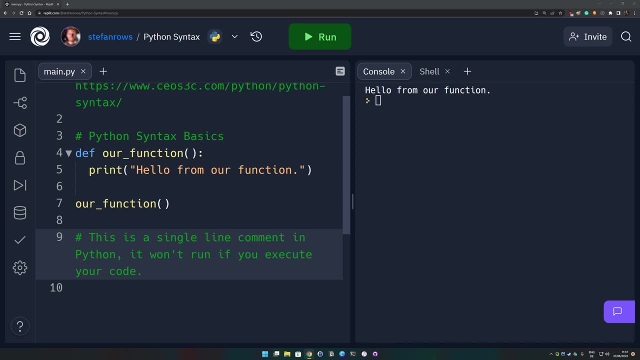 or so-called string literals. So if you're declaring strings in Python, you have a bunch of options here You can declare a string. Let's first create a variable here. Let's call it ourString. This is how you declare a variable in Python. if you haven't seen that before, 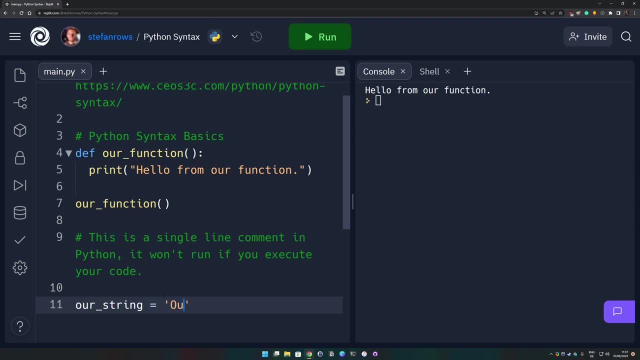 And we can go and we can declare a string by using string. We can call that ourString. But we can also use double quotes instead of single quotes and it doesn't really make a difference. We just have to make sure to not use too many quotes. 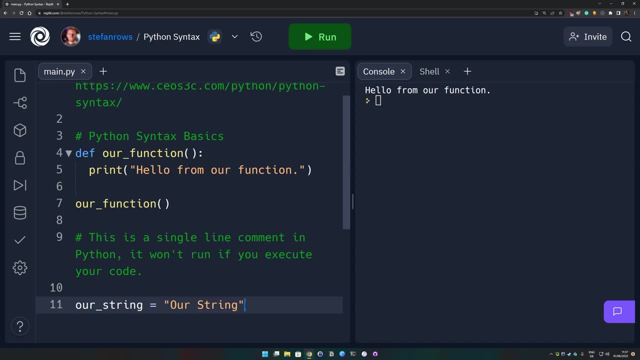 So we only use double quotes for this And this will work just the same. And to prove that to you, let's just print it out here: Print ourString, And we quickly comment out that function call here. And this is also a way how you can just comment out code. 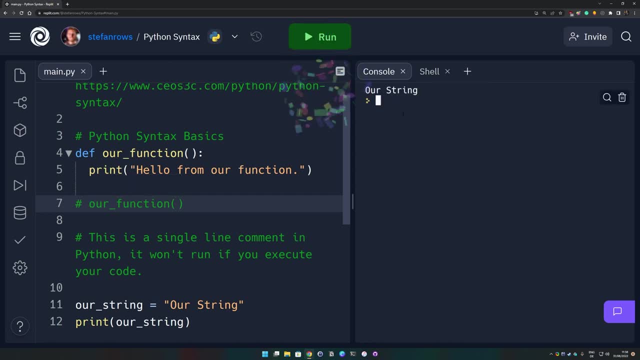 But you don't want to run when you're testing something, So this is printing out our string. Let's put that back to single quotes to demonstrate that it's actually working. And then if you print that out, that prints out exactly the same. 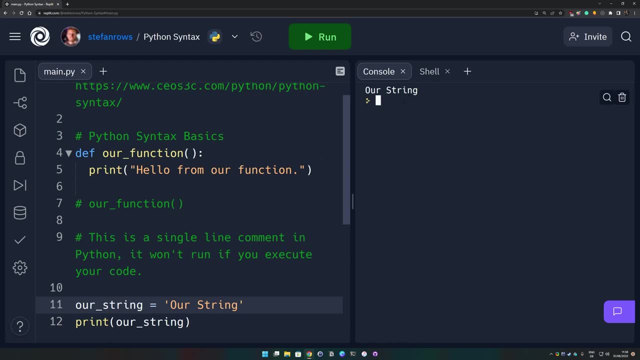 We can also use triple single quotes or triple double quotes, But it's crucial that you always start and end a string by using the same type of quotes. For example, if you start your string with a double quote, You can't end it with a single quote. 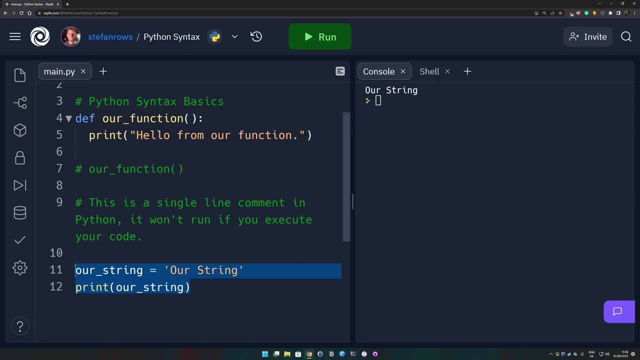 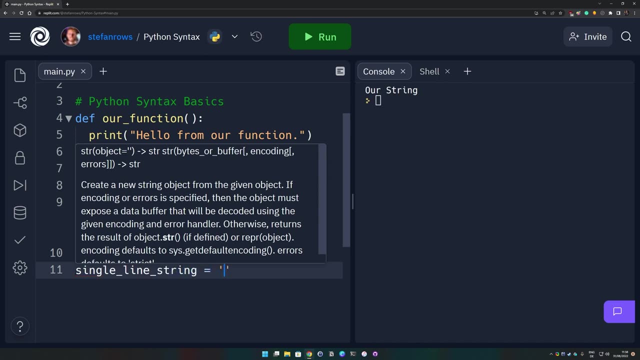 So let's look at some examples below to better understand that whole concept. Let's create a single line string here and give that single quotes, And then we say: this is a single line string using single quotes. So this is our single line. Now we print it all out in the end. 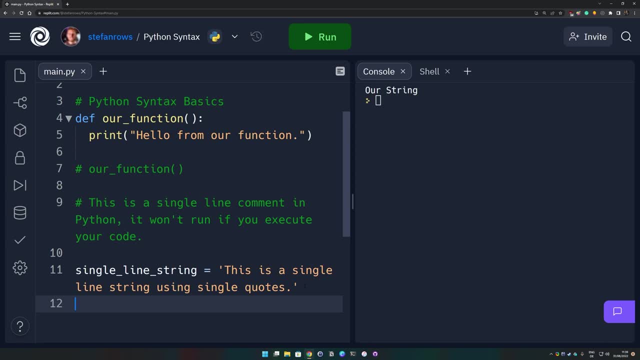 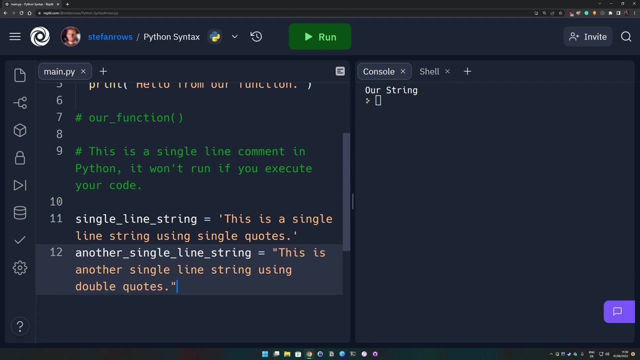 Let's create a bunch of strings that we can look at the output also. Then we create another single line string And we equal that to. this is another single line string using double quotes. This is our second string And then we create a multi line string. 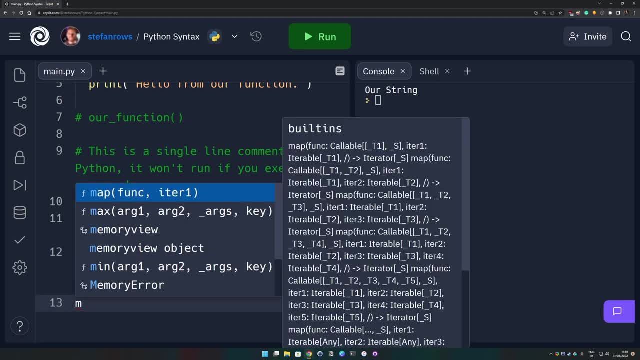 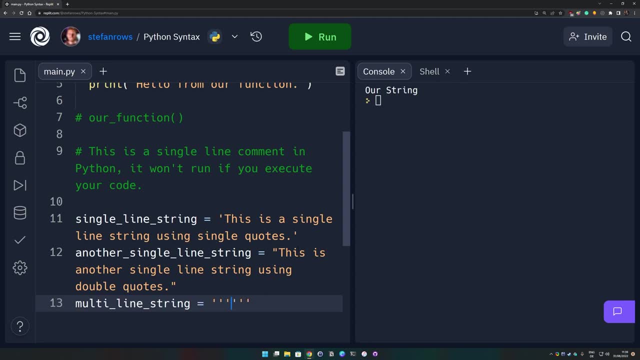 So to create multi line strings, we are going to use triple single quotes or triple double quotes. We do multi line string Equals And then we do triple quotes, And if you just hit the button three times, it will automatically create triple quotes. 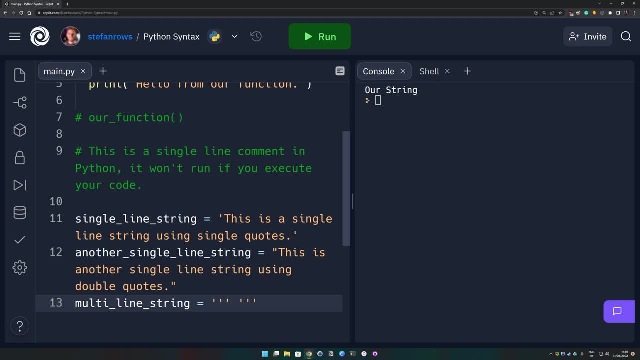 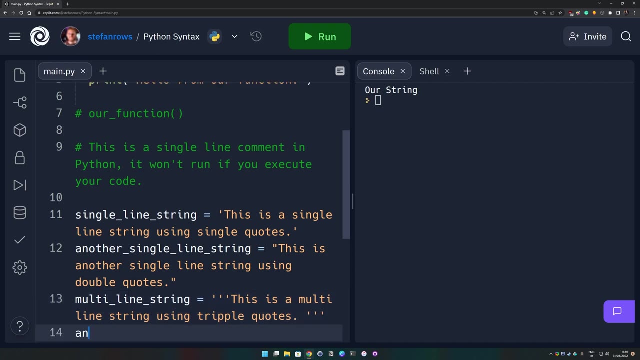 here. So you can see we have six quotes all together And now we can go ahead and we can do. this is a multi line string using triple quotes. Now let's create a final one that we call another multi Line String And equal that to three double quotes. 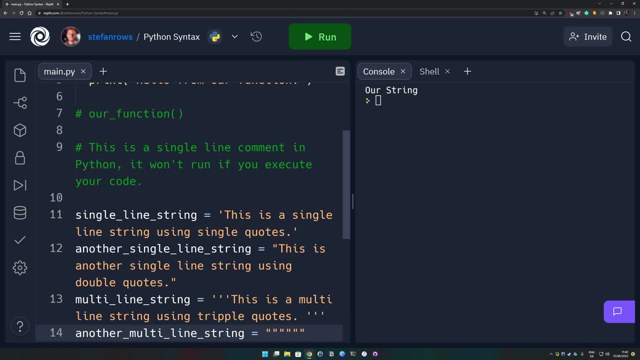 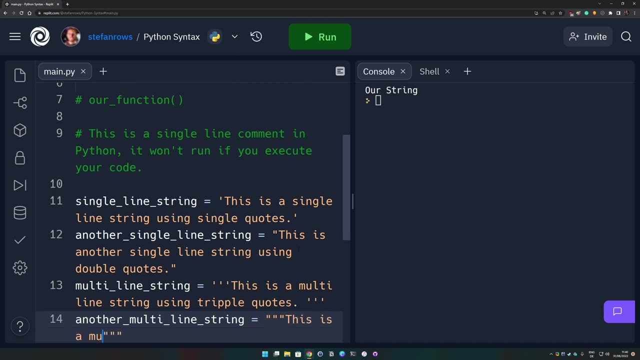 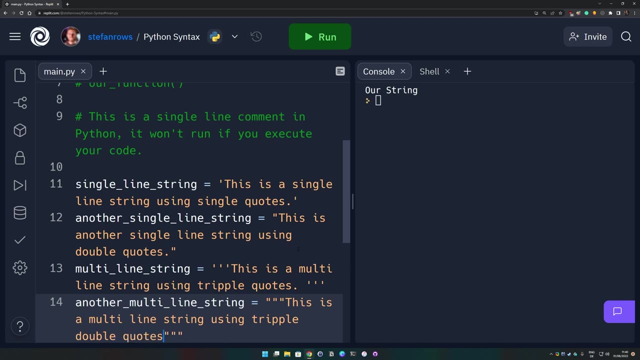 Triple quotes: Yeah, Two. Okay, Now I'm getting confused. It's six triple, Six double quotes. And then we do. this is a multi line string using triple double. Oh my God, Triple double quotes. Okay, There we go. 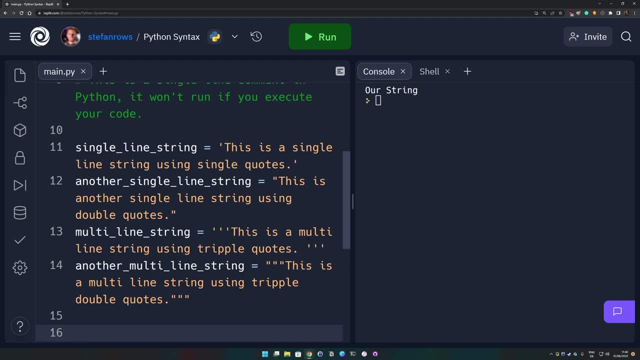 Now, if you want to print out all of that, we can simply do that by using a print statement. So we do print single line string and then we just copy that a bunch of times, So we don't always need to reprint it or retype it. 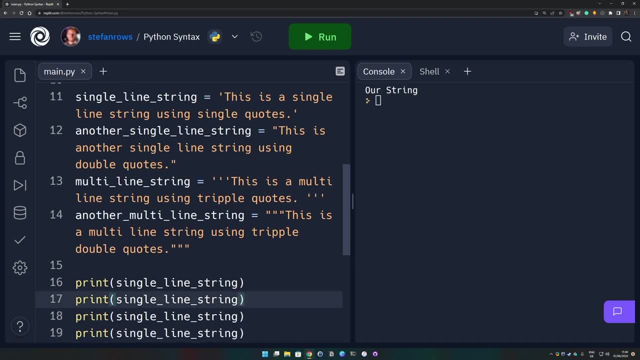 We do that four times and we do. it's the other one called another single line string, And then we do multi line string, multi line string, And then we do Another Multi Line String, Another Multi Line String. 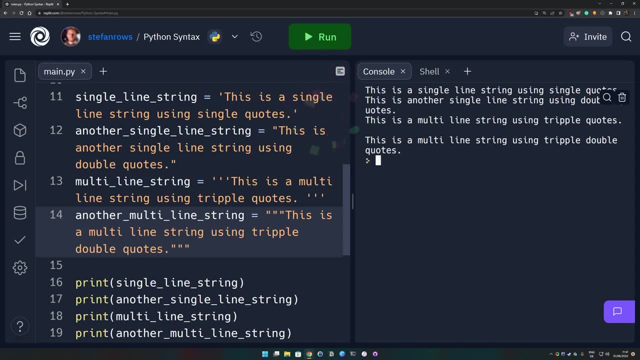 There we go. So if you print all of that out, we get the result and you immediately can see that there's actually a space between these and there is no space in here. So why do we actually use multi line strings? We use multi line strings if we want to have some space in between the lines that we are. 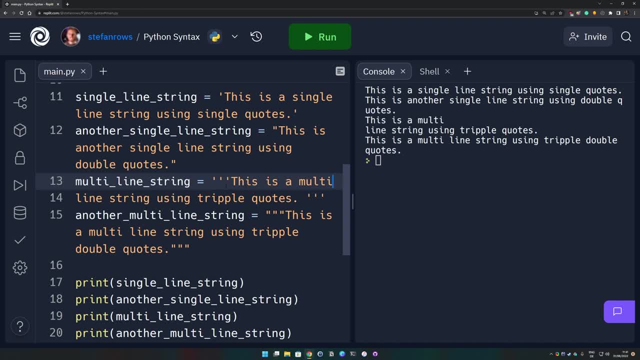 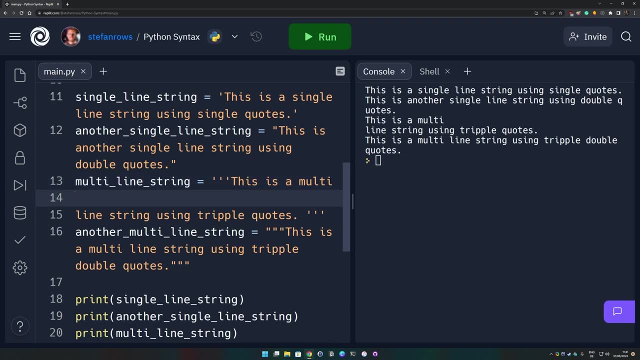 printing. And this is exactly what we are seeing here Now. if we go to the triple single quotes Line of code and we say this is a multi line string using triple quotes and we just hit enter and we gifted some space in between and then we run the code, then you can actually 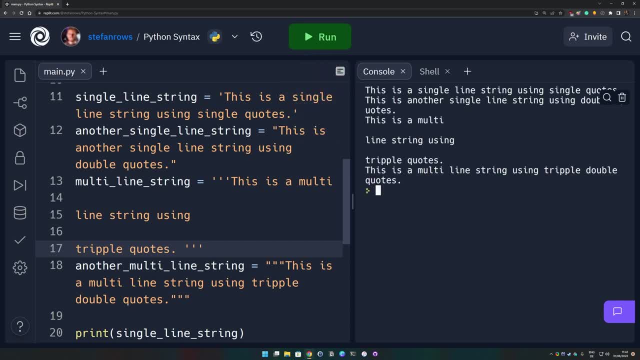 see that those lines have actually been separated. So this is not the case if we do that in a single line string. So if we would do that here, it would already give us an error, because it recognizes that it's only single quotes, or single double quotes in that case, and it doesn't allow us to hit. 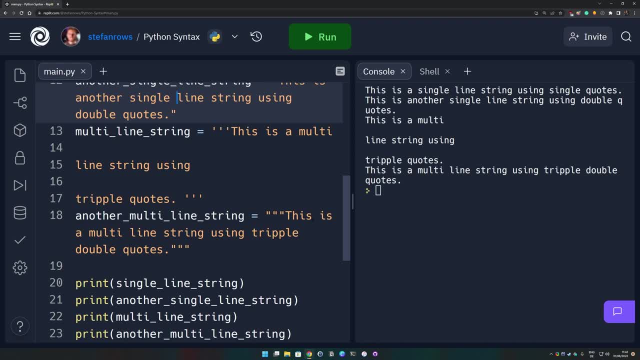 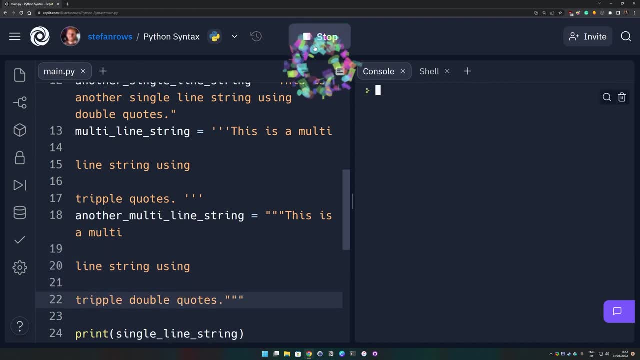 the enter button. So the same is true for the triple double quotes here. We can also use the enter key here to create some space between the print statements, And if we look at that again you can see that that is actually printing out with space. 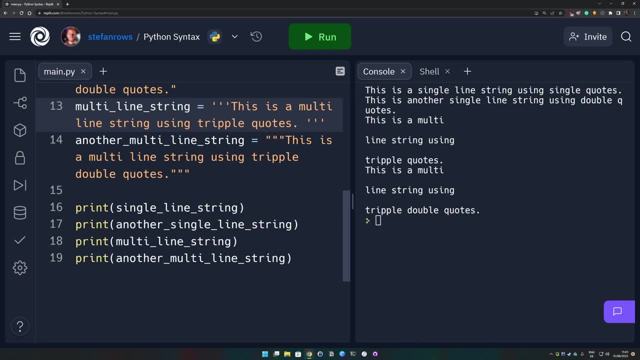 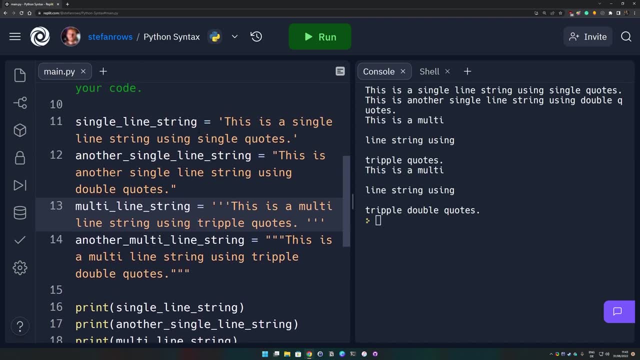 in between. So to summarize that we use multi line strings to print out spaces between our lines And we use usually single single line strings using single quotes or double quotes when we just want to print out a single line with any space in between. So this is also an essential part of Python syntax. 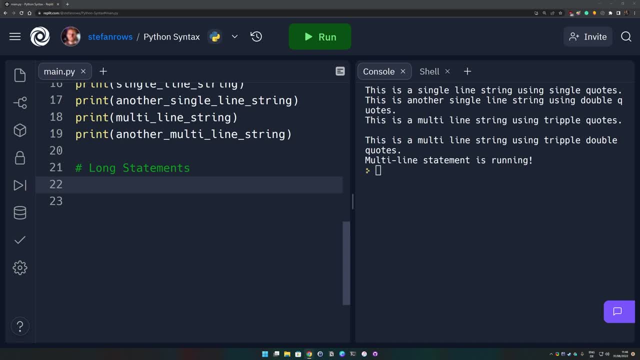 So the next thing we want to take a brief look at are so-called long statements. In the Python programming language, it is sometimes required to use longer statements that need to be separated for better readability, and we can utilize a backslash to achieve that. So what I'm talking about here is, if you write a very long statement that would exceed the 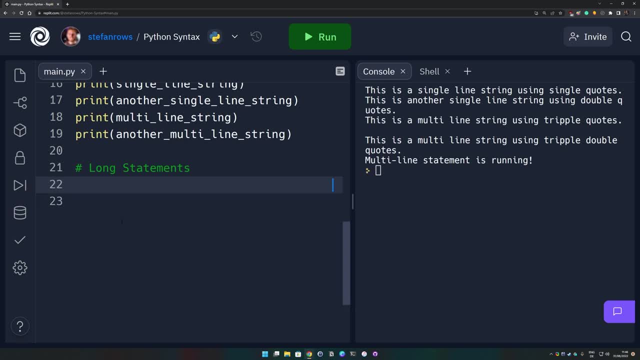 line here And in your code editor you maybe would not see the line anymore because it got too long. Then we can utilize a backslash to separate that line, much like in those multi line strings. So to do that I create a simple if statement here to demonstrate that for you. 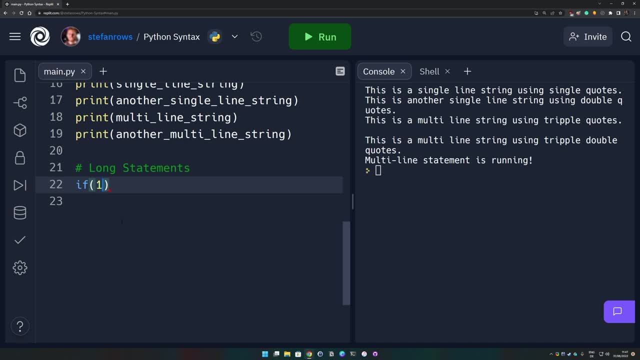 Don't worry about the logic here. it doesn't, it's not necessary, It's just about the syntax. So if we do a simple statement here where we check if some numbers are equal to another or bigger or smaller than the other one, We can just do that by creating a simple. 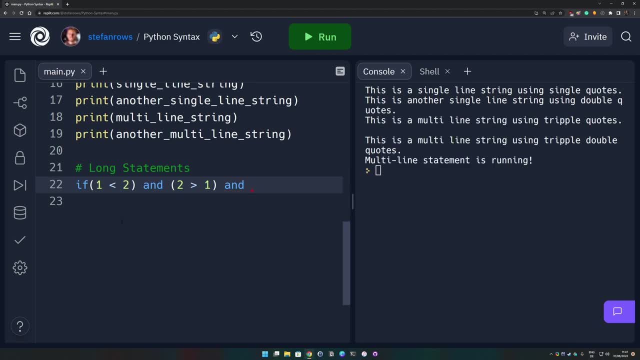 Number game here, and then we do another end statement. and now let's say, if we want to continue this logic on the next line, we can do a backslash here, and then we press enter. Now we need to indent our code here a little bit for that to work. and then we do another. 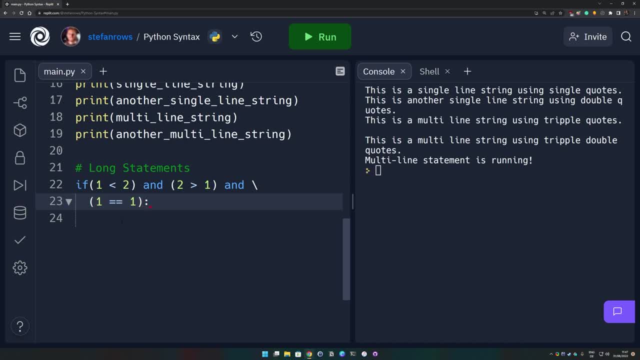 condition down here and then we do a colon at the end and then we want to print out something. if that all, if all these conditions are true, So we do multi Line Statement. End Line Is Running And let's actually check if that works. 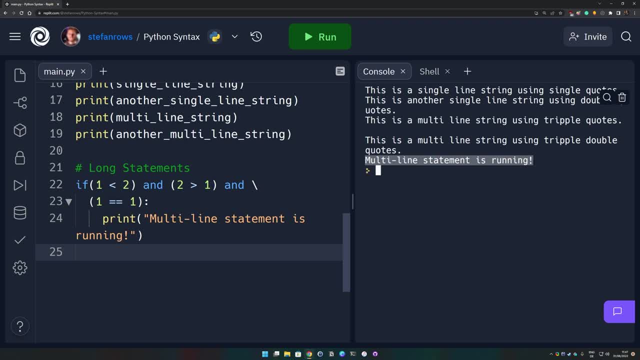 And it is working. The multi Line Statement Is Running. This is good to know because if you run a very long statement, if you write very long statements here, then you might run out of space and it gets hard to read. so separating them. 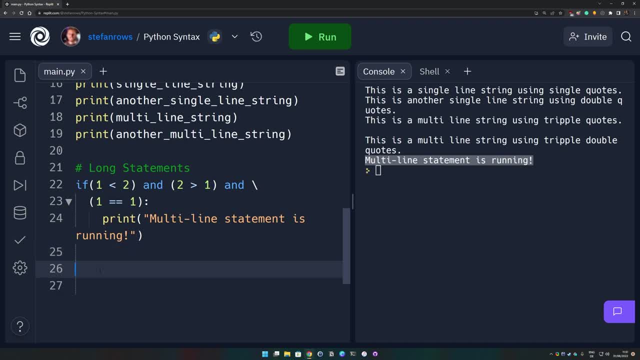 in different lines makes it a lot easier. The last thing I want to quickly talk about when it comes to understanding a basic Python syntax is casing. So by casing I mean how do we actually write our variable names, and so on and so forth? 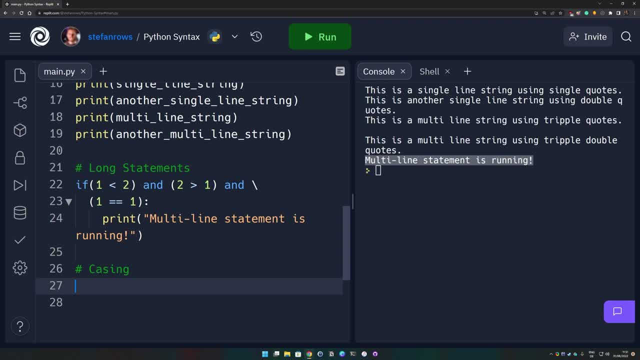 So we do casing and then we look at some examples. So while sticking to casing isn't mandatory for your code to work, it is highly recommended to stick with the recommended casing standards for Python according to PEP 8.. And those standards are variables. functions, methods and modules are written in snake. 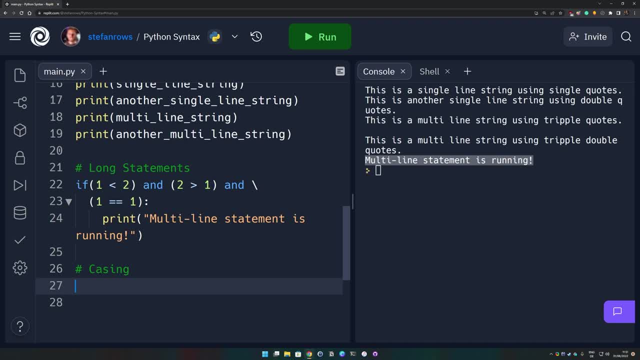 case, classes are written in Pascal case and constants are written in capitalized snake case. We highly recommend sticking to these guidelines, which helps tremendously with making your code better readable, both for you and anyone who works with you. Let's take a quick look at some of the examples below, then you better understand what I'm. 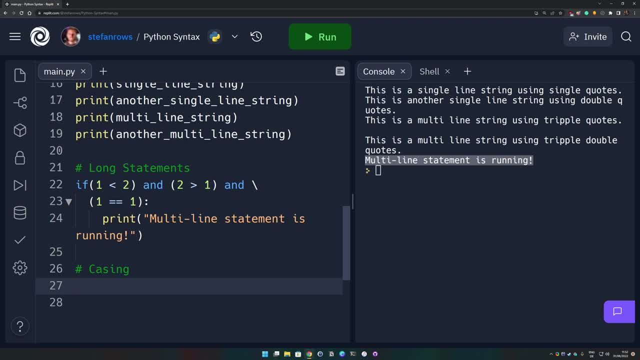 actually talking about. So camel case means capitalizing the first letter of each word, except the first one, and removing all spaces. We do Python syntax and equal that to a string. That's camel case. So this is how camel case looks like. That's actually not used in Python a lot. 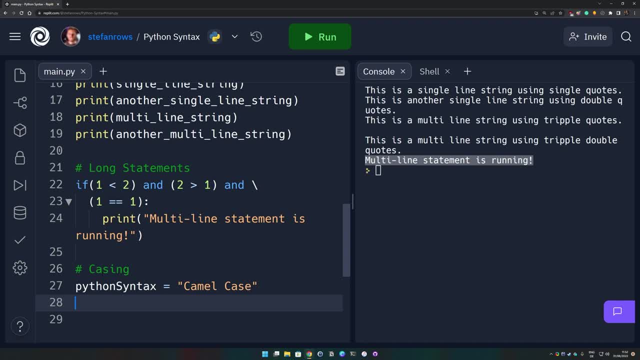 Very rarely I see that and it's not recommended in the style guide. So this is just for you to understand what camel case is. The next one is important. That's Pascal case, Capitalizing all first letters and removing all spaces. So we do Python syntax. 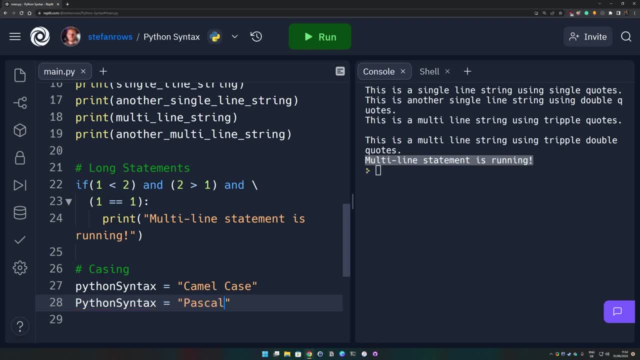 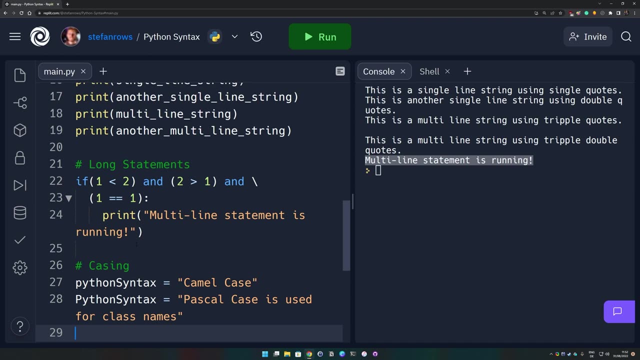 It would look like this, And then we say: it's Pascal case. Okay, So Pascal case is only used for class names in Python. Okay, So we got that. The next one is snake case. Snake case is written like this Python syntax: 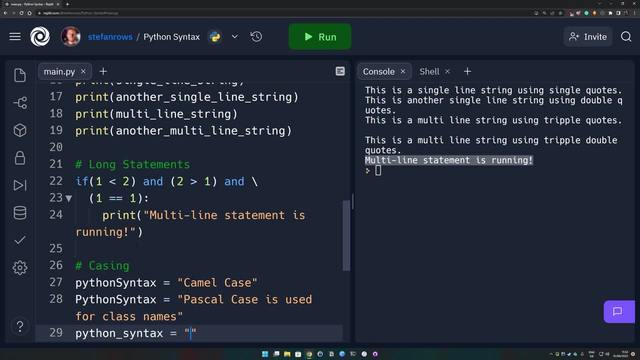 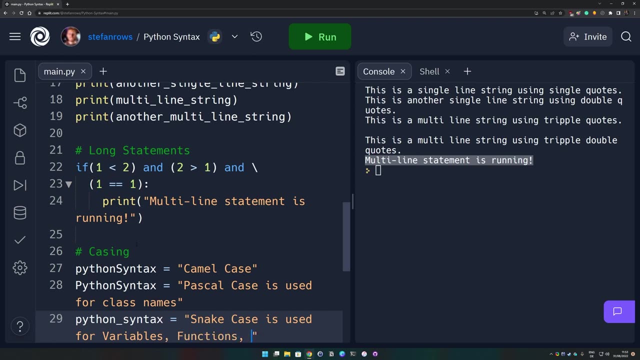 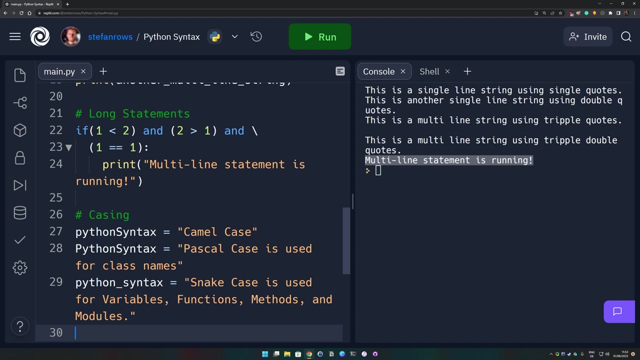 And then we equal that to snake Snake case is used for variables, functions, methods and modules. Is used for variables, functions, Methods, Methods, Modules. Okay, And the last one is capitalized snake case. So we do Python syntax. 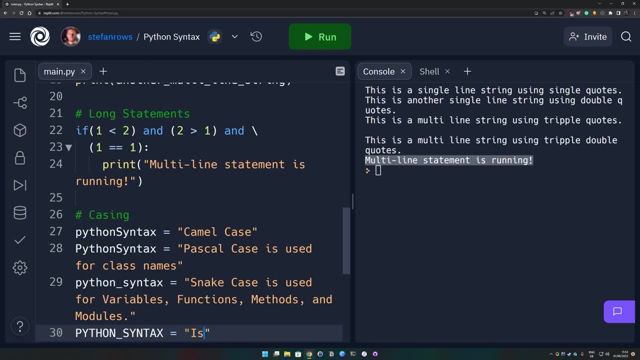 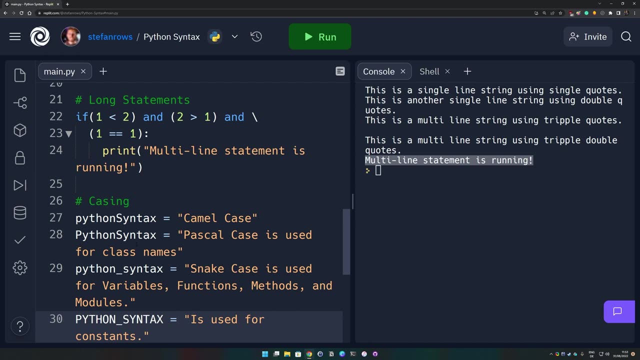 And capitalized is used for constants Is used for constants. Now you don't need to worry about what constants are. We have another article in the video. when you want to learn more about constants, I'll link it in the video description below And you will learn everything you need to know about Python if you just check out our Python category on seoseccom. 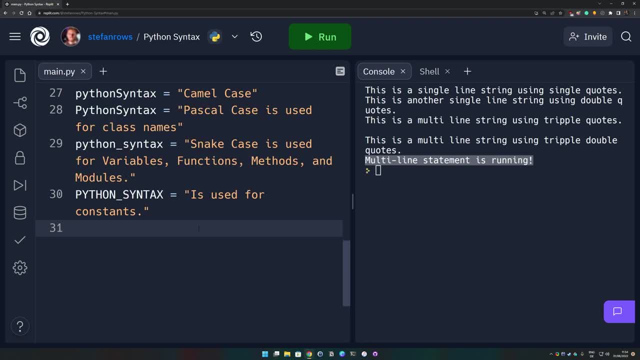 So, to summarize what you have learned today, Python code is indented with spaces or tabs. That was the first thing we were talking about. In Python, we use snake case for variables, functions, methods and modules. We use Pascal case for classes. 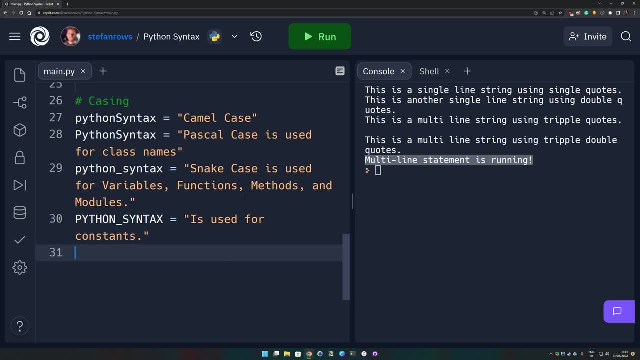 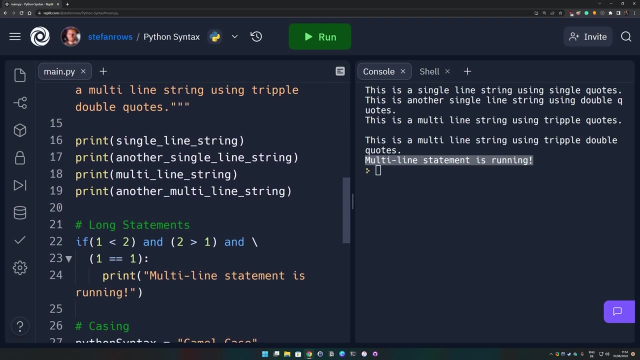 We use capitalized snake case for constants, as you just have seen here. We can separate long statements with the use of a backslash. We can use different types of quotes for string literals- That's what you have seen here. And finally, we can use hashtags for writing comments. 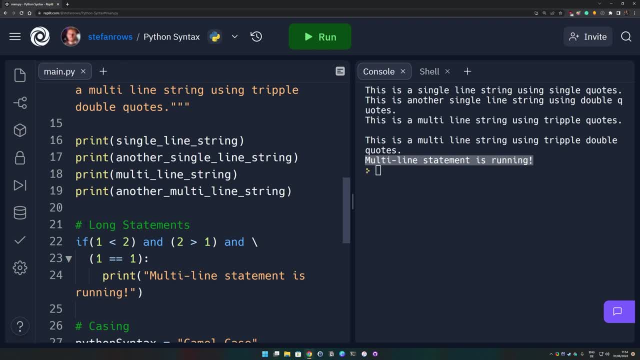 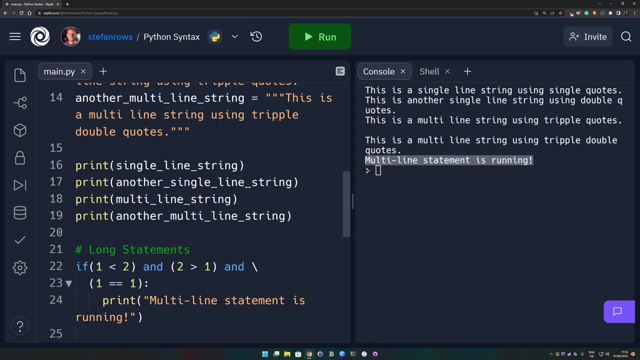 Now, if you want to learn more about Python, we highly recommend checking out our Python category on seoseccom. If you click on learn on the top navigation bar and click on Python, there are all of our Python tutorials, And all of our Python tutorials usually come with a corresponding replit that you can directly code with us.